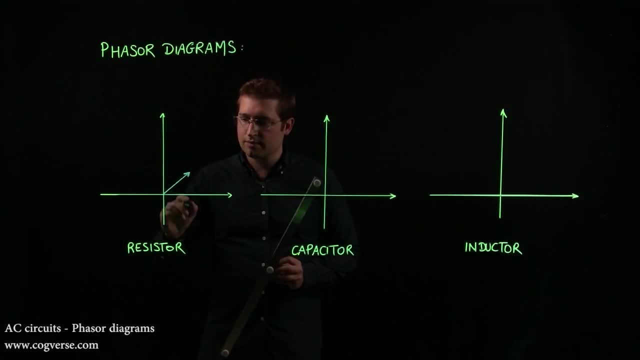 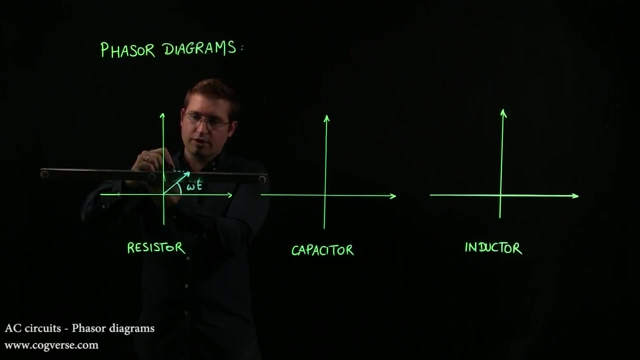 With a length equal to I naught, and an angle here that is omega t. After a certain amount of time, after t seconds, because this phasor rotates at angular speed, omega, this angle is omega t, And that means, of course, that if we look at this projection here, we get: 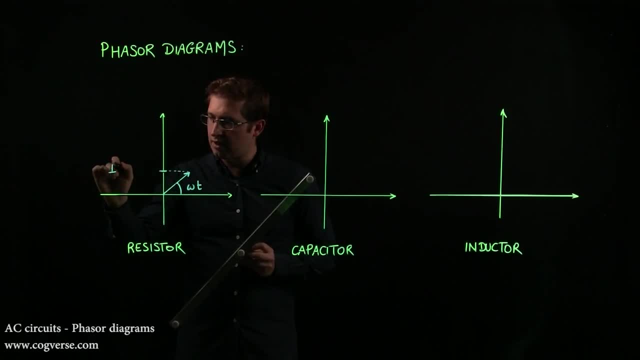 I naught the length of the vector sine omega t. So this here is really going to give us the current at time t. So that's for the current. We know that the voltage is in phase with the current. for a resistor. 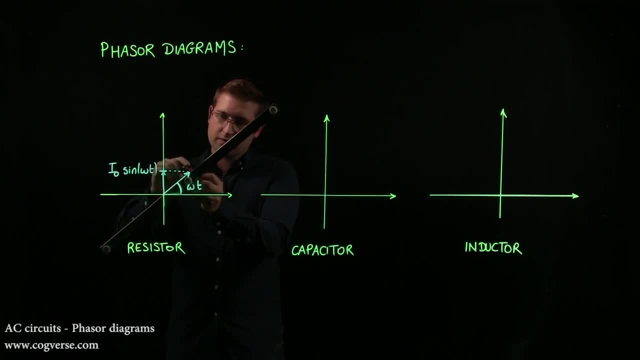 And so we're going to have a phasor that looks like this: For the voltage, it's going to have a length, V naught, and the same angle, omega t, which means that here we get a quantity that is V naught, sine omega t. 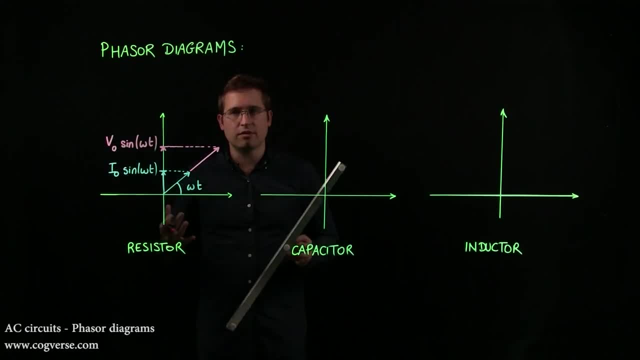 And because they're aligned, we know that I of t and V of t are in phase. So it's a very visual representation of these equations that we've just derived, And the nice thing is that it allows to add voltages or currents together, using vector addition or vector subtraction. 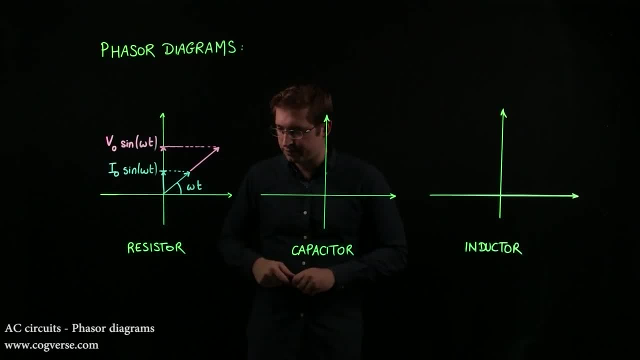 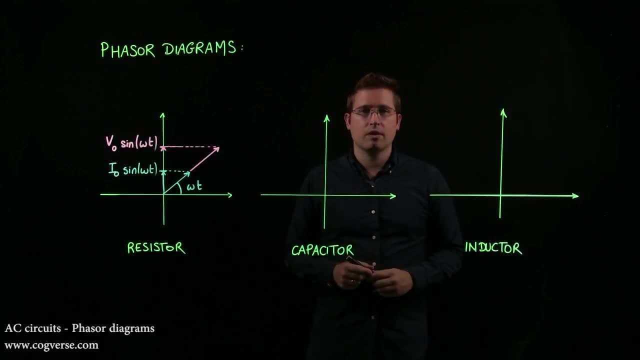 So it's very easy to manipulate phasors once you have them. So as for the resistor, let's do the capacitor. For the capacitor, we said that the current leads by pi over 2. So the current is going to have to be ahead of our voltage. 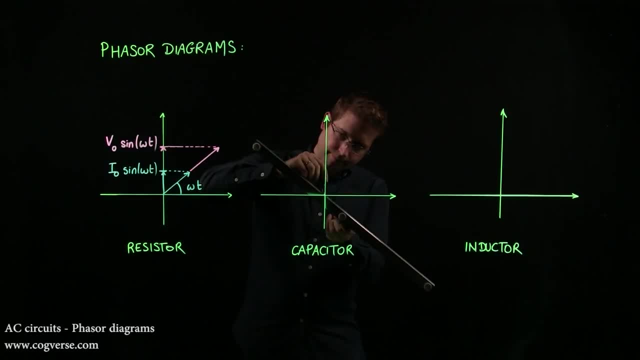 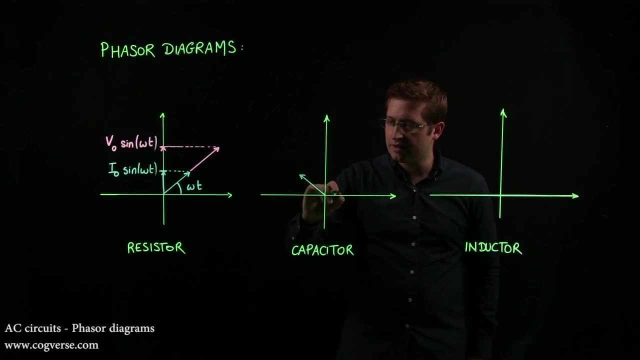 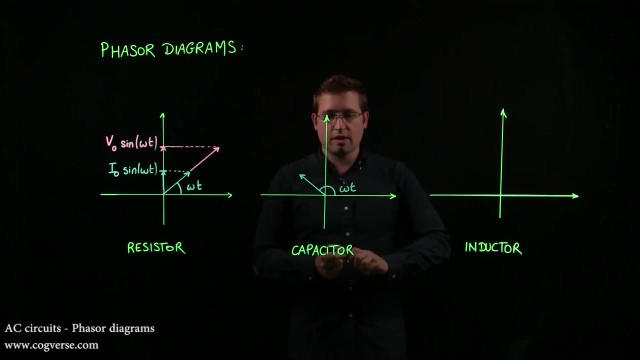 So let's draw the current like this, And it has a magnitude. I naught, and this angle here is going to be omega t. Now, if the voltage is behind, as in if the current leads, then the voltage is behind by pi over 2, and that's 90 degrees.